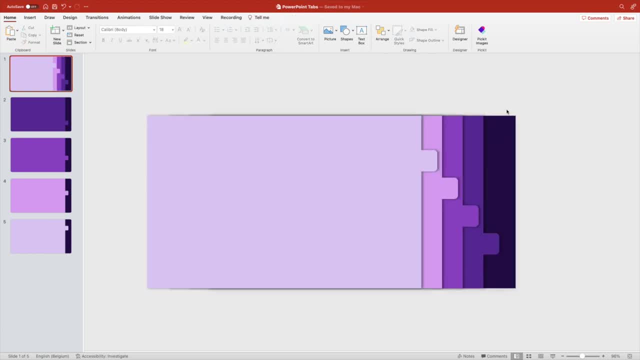 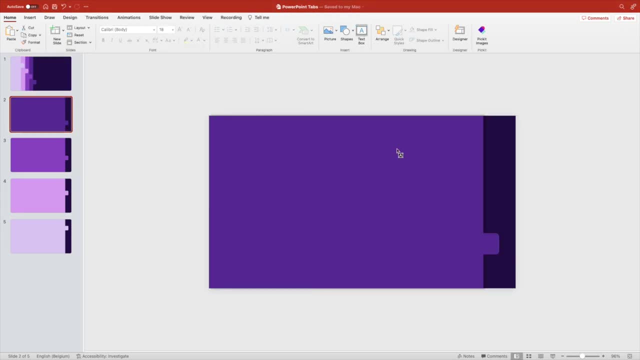 last one, perfect, and now we can select everything and move it to the left. so this is the, the final result that we're looking for. now. we want to create all the content on the different tabs, so let's add a large number- 1, 2, 3 & 4- make. 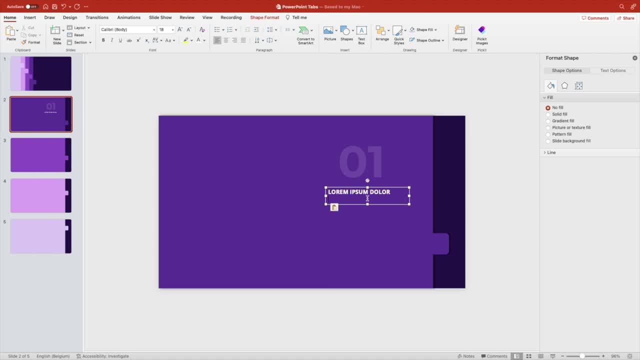 it a little bit more transparent, and that way it's a little bit more subtle. add a title and some dummy text. you want to work on the right side of the slide, so don't just fill up the entire tab, but you want to work on, let's say, the right. 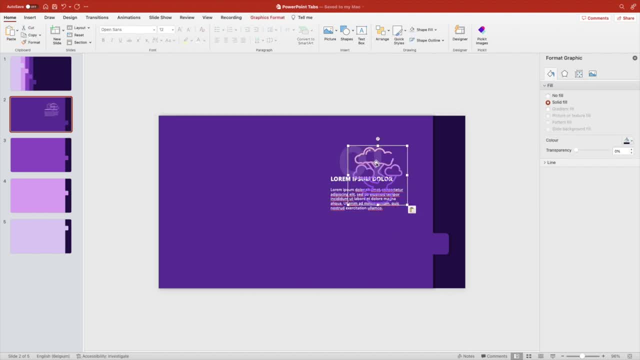 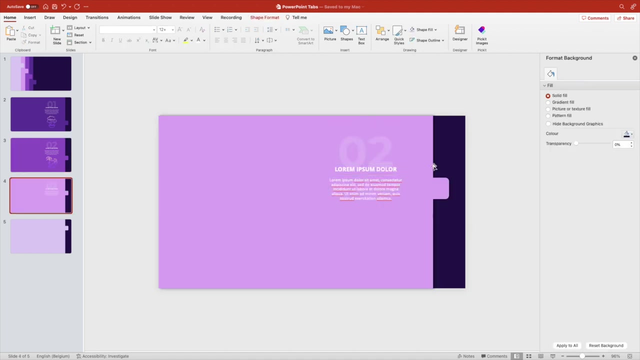 half of the slides because we're going to pull them out and overlay the tabs to the left and I can select everything and center it align to Center. now we can copy this to the second slide, change the number to 2 and create or add a new icon. and do the same for the other pages, the third one: add a new. 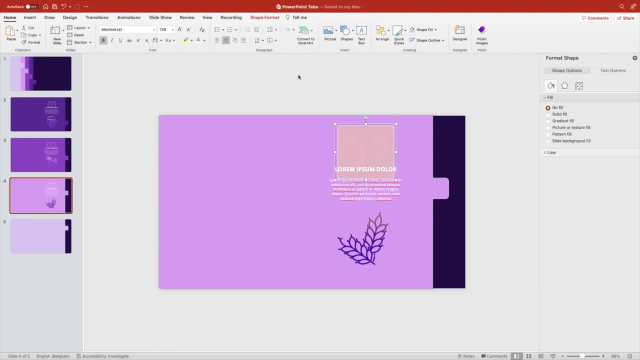 icon and the text seems to be a little bit lighter. so let's change the color, make it something purple, that way it stands out a little bit more, and then copy it one last time for the fourth slide. that looks good, and change the icon. now we want to add the numbers to the slides. 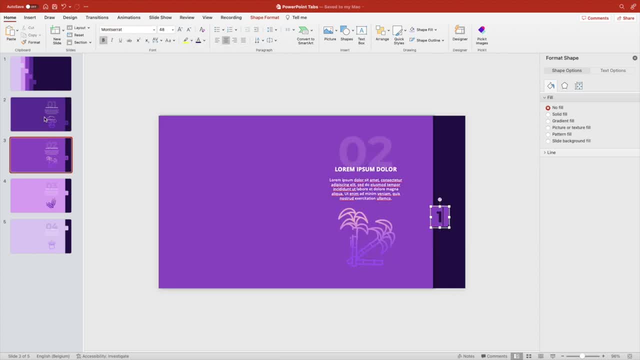 so add them with the color of the previous layer, so the firm on the first layer. we'll look at the background and then we'll make the color a little bit lighter as we go along. I change the numbers here from 4 to 1 and then we'll. 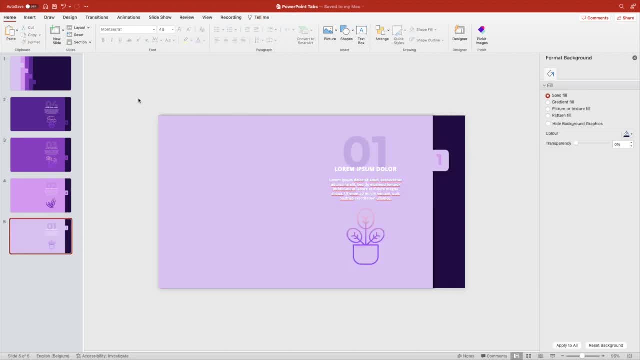 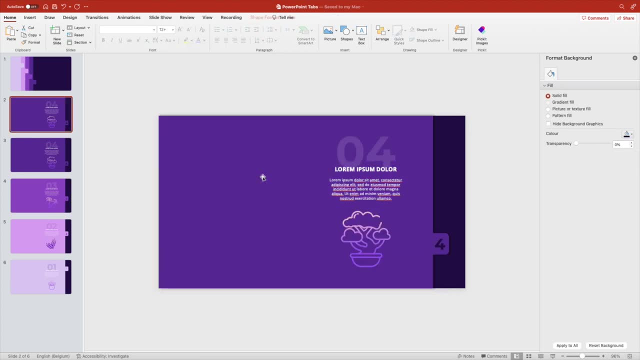 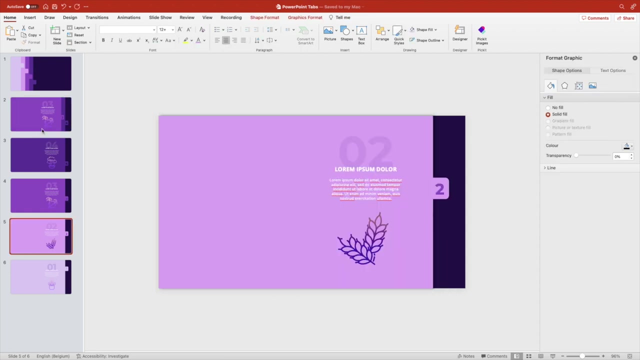 add a new one so that 4 comes at the bottom and 1 is at the top. that feels a bit more natural. group everything together and then create a copy of the first slide and just overlay all the different stacks, shift them to the left a little bit. so number three goes on, number four and then number two goes on.